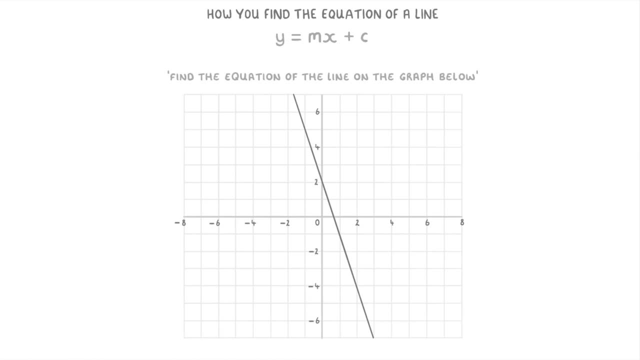 the line on this graph. The easiest thing to spot is that the line crosses the y-axis at y equals 2., Which tells us that c must be 2.. The gradient, though, is a bit trickier and there's a few different ways to find it, but in this video we're going to use the equation. change in y. 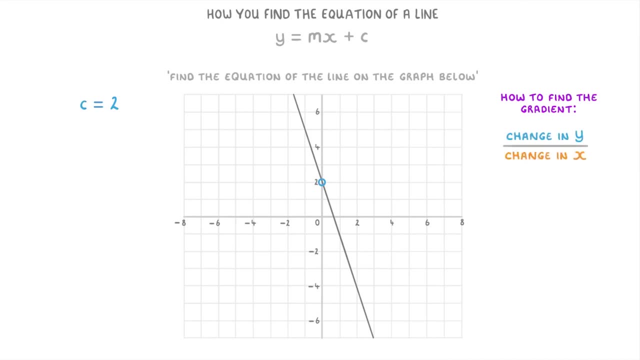 divided by change in x, which just means how much the y values change by, divided by how much the x values change by. So, to use this, we pick any two points along the line, for example- these two label them points on the line- and then we'll use the equation to find the gradient of the line. 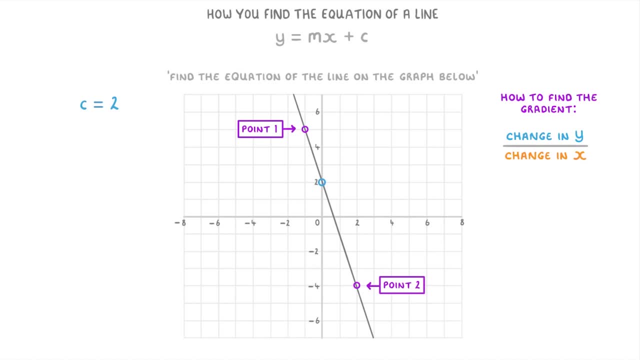 So to use this, we pick any two points along the line, for example these two, label them points on the line, and plug those values into the equation, Point 1 and point 2. And then draw vertical and horizontal arrows between them so that we can form a right angled triangle. 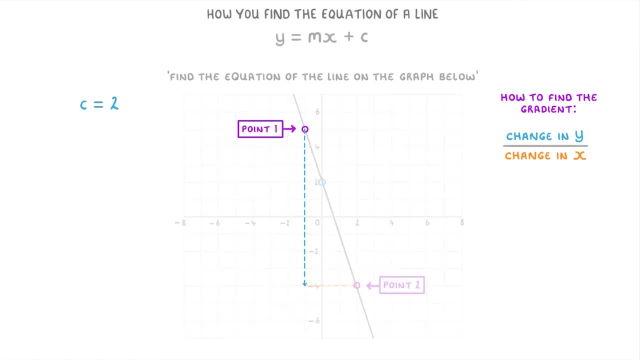 Then to find our change in y, we can see that the vertical arrow goes from positive 5 all the way down to negative 4, which is a change of minus 9.. So our change in y is minus 9.. In the same way, the horizontal arrow goes from x equals negative 1. 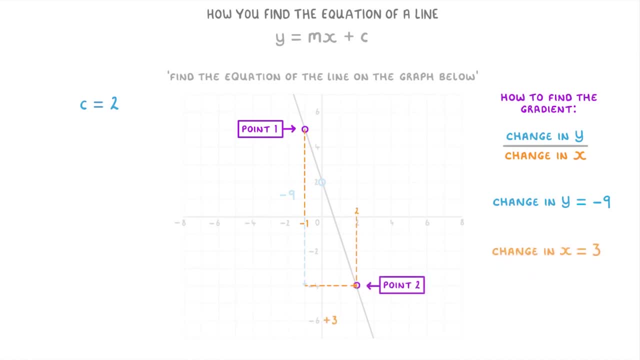 1 over to x equals 2,, which gives us a change in x of positive 3.. This means that to find our gradient, we just do the change in y of minus 9 divided by the change in x of 3, which. 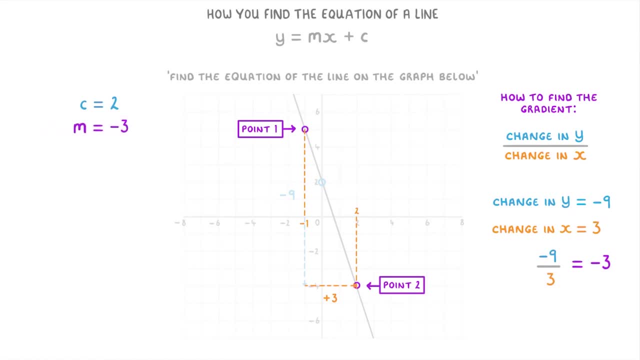 will give us negative 3.. So m in our equation is minus 3.. And so, to finish, we just take our equation: y equals mx plus c and plug in the minus 3 as m and the 2 as c, which 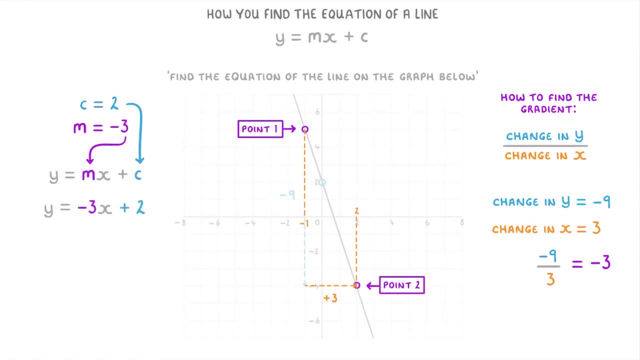 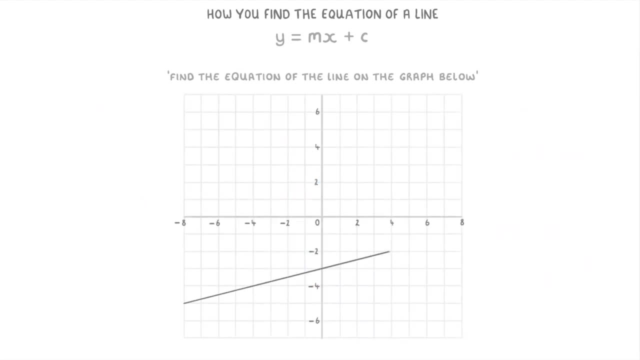 will give us y equals minus 3x plus 2 as the equation of our line. Before we finish, let's try the same thing for this one. The first thing you want to do with all of these questions is write out y equals mx plus c, because that's the general format that we're going to need. 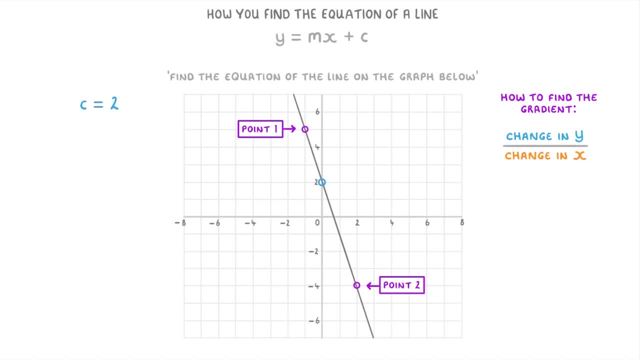 So let's start with the equation of the line crossing the y-axis at y equals 2.. And then draw vertical and horizontal arrows between them so that we can form a right angled triangle. Then, to find our change in y, we can see that the vertical arrow goes from positive 5. 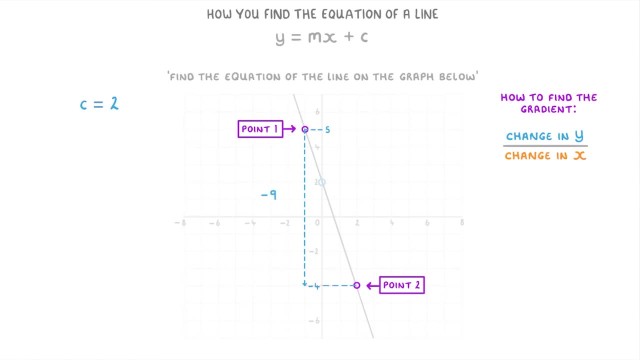 all the way down to negative 4,, which is a change of minus 9.. So our change in y is minus 9.. In the same way, the horizontal arrow goes from x equals negative 1 over to x equals negative 2.. 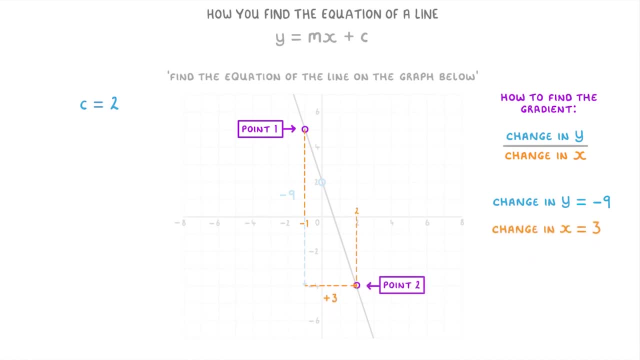 Which gives us a change in x of positive 3.. This means that to find our gradient we just do the change in y of minus 9, divided by the change in x of 3, which will give us negative 3.. So m in our equation is minus 3.. 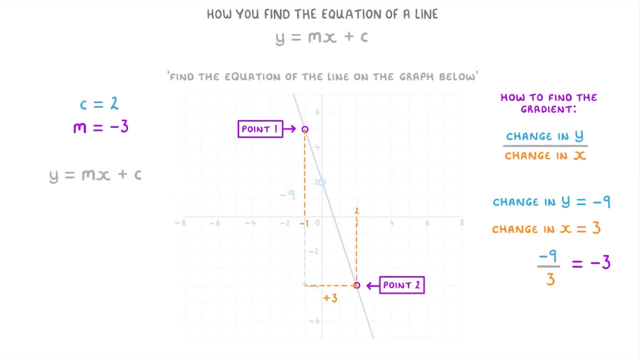 And so, to finish, we just take our equation y equals mx plus c and plug in the minus 3 as m and the 2 as c, Which will give us y equals minus 3x plus 2 as the equation of our line. 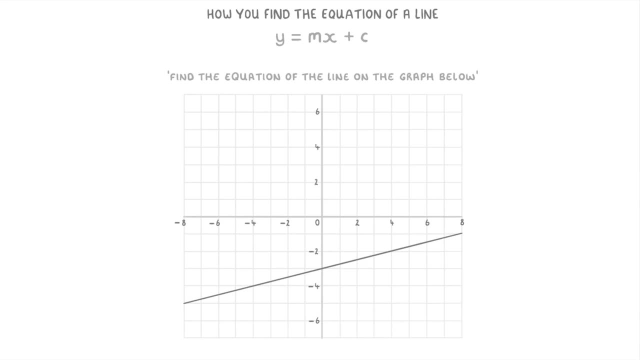 Before we finish, let's try the same thing for this one. The first thing you want to do with all of these questions is write out y equals mx plus c, because that's the general format that we're going to try and put our equation into. 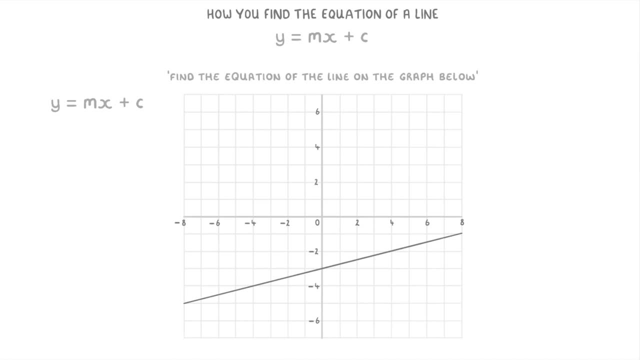 Then to find c, we need to look for the y-intercept which is down here at negative 3.. So you know that c is negative 3.. Next you need to find the gradient which requires us to find the change in y. 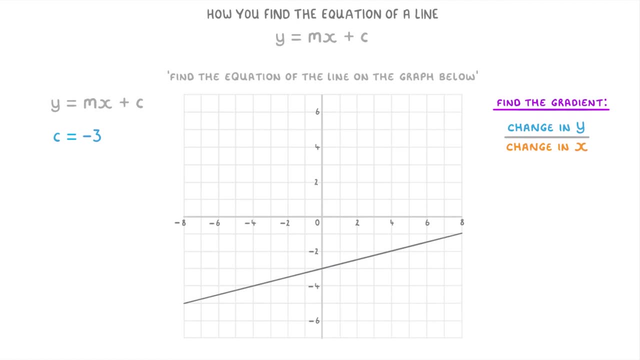 and divide it by the change in x. So for that you need to pick two points along the line, for example 0, negative 3, and 4, negative 2,, label them both and then draw the triangle thing. 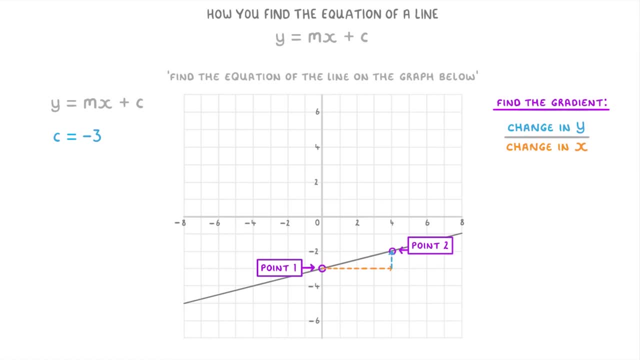 So if we go from point 1 to point 2, and start with the y's, we can see that we've gone up by 1, so our change in y is just 1.. And then if we look at the x values, we can see that we've gone along by 4,.